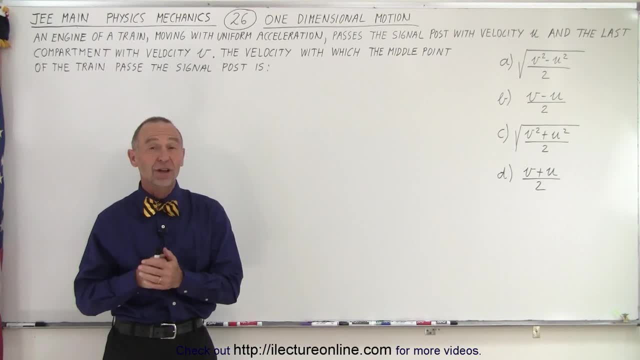 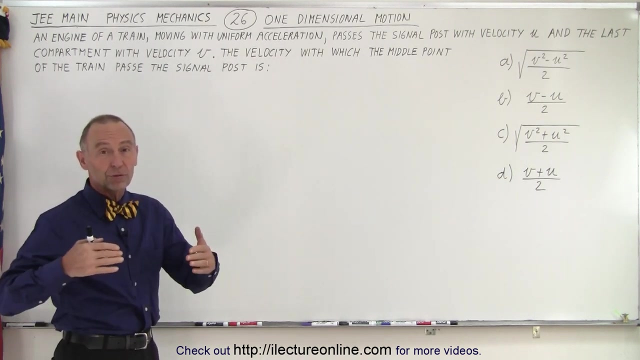 Welcome to our lecture online Here. our next problem on the JEE main physics test. It looks pretty easy on the surface. Is it easy to accomplish? Is it easy to work it out? Well, let's find out. It deals with one-dimensional motion, so that's one of the most 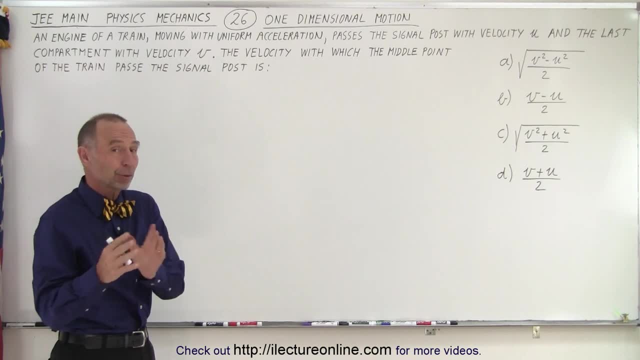 principal concepts that you'll encounter in any physics books. right at the beginning of the book The problem says an engine of a train moving with uniform acceleration passes a single post with velocity u and the last compartment with velocity v, The velocity at which the middle 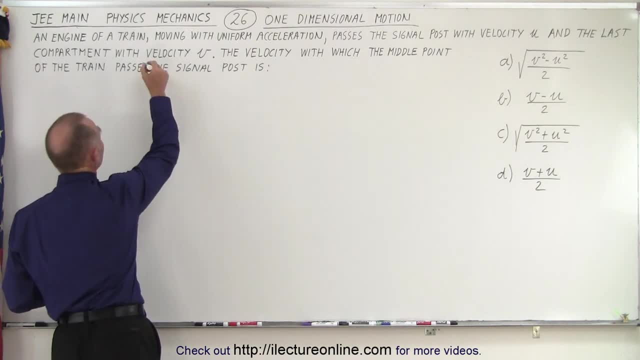 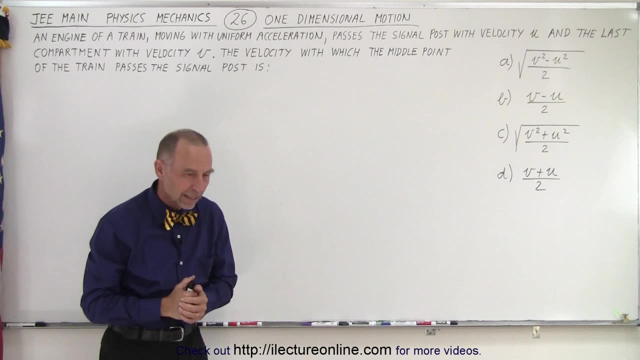 point of the train passes- and I think I'm missing an s- there passes a single post is, and they give us four possible answers. Now the reason why it's deceiving is you would say, well, wait a minute. if the beginning of the train passes the post with velocity u and the end of the train with velocity 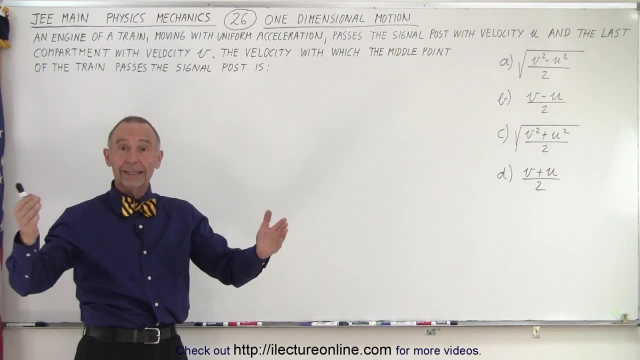 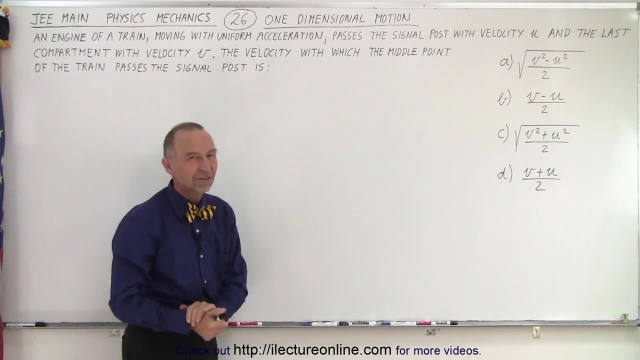 v, and now we want to know the velocity in the middle of the train. is it simply the average? So the average would simply be the sum of the two divided by two. Answer d, But it turns out that's not the correct answer because it's not a linear thing. There's uniform acceleration. 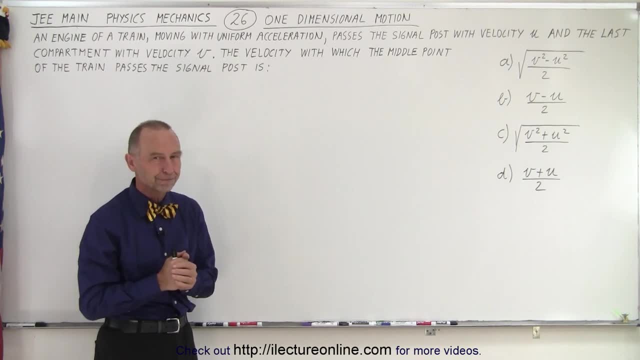 and because of that we can't use that technique to solve the problem. Instead, we're going to have to use the equations of kinematics, and in particular the three equations of kinematics. So just for getting us oriented to what the principles are. 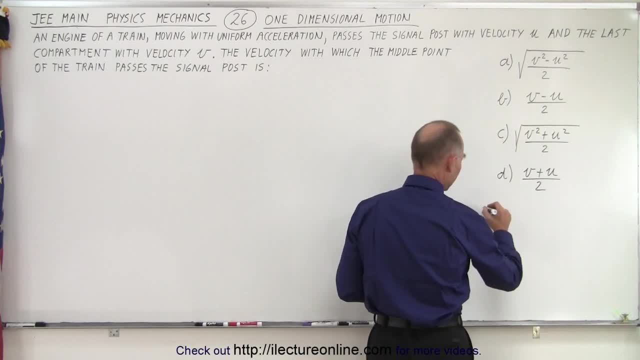 here let's write down the three equations of kinematics. The first one is x equals x sub naught plus v sub naught times t plus one half a t squared. The second equation is: v equals v sub naught plus a t. and the third equation is: v squared equals v initial squared. 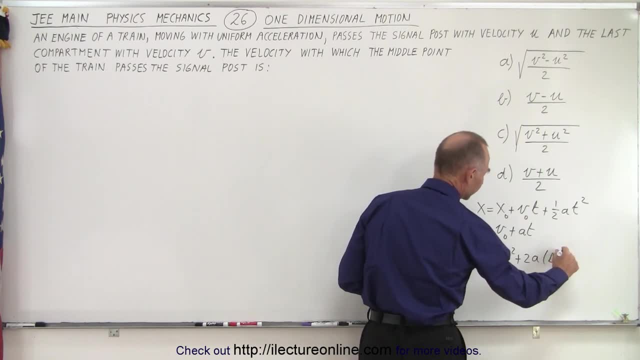 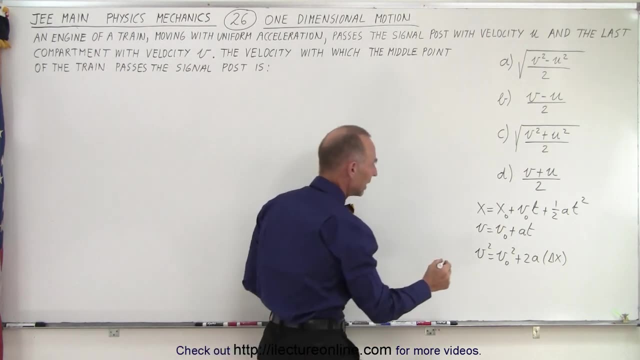 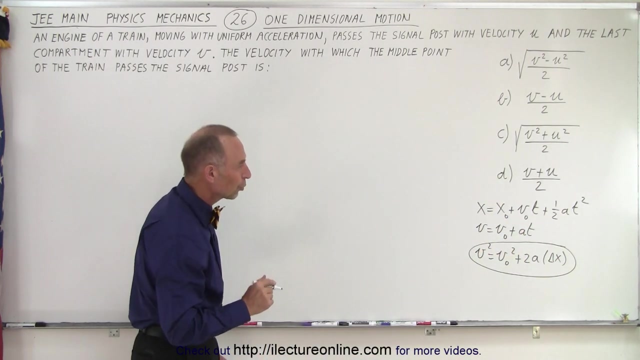 plus two a times delta x, And the equation that we should be using out of those three, since we don't know anything about the time, is equation number three. That's going to be the equation that's going to help us solve this problem. Now notice, we're trying to find the velocity of the middle of the train. with respect, 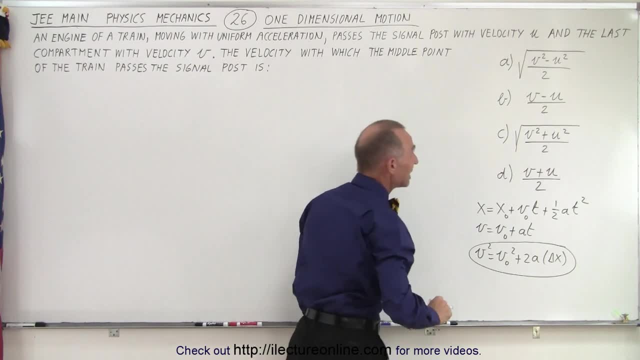 to the velocity in the beginning and the end in terms of v and u, and all the answers are, of course, in terms of v and u, So let's go ahead and apply this equation. So v squared, that's the final velocity squared. Well, what we want to do now is the velocity in the middle, So let's use v. 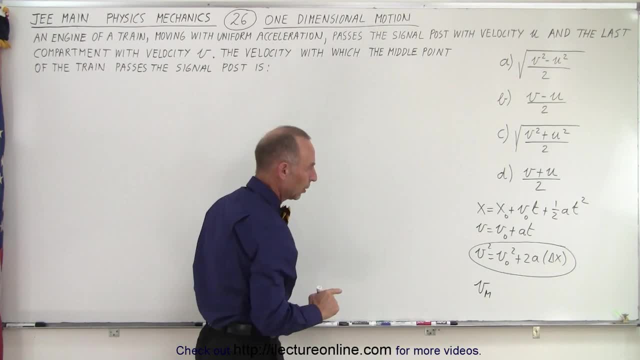 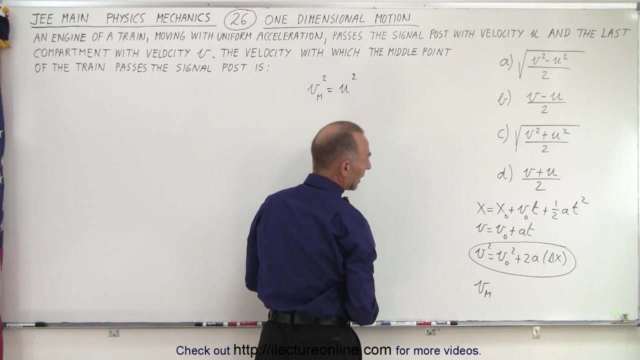 sub m as the velocity in the middle, to help us out. So that would be, so to speak, the final velocity. So here we can write: velocity of the middle of the train squared is equal to the initial velocity squared. Well, we'll start with u? u, squared and plus two times acceleration times, the amount of. 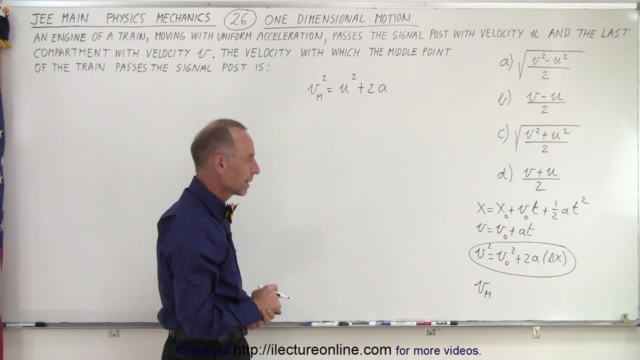 the length of the train that has gone by. Well, the length of the train that has gone by would be l over two. All right, that should work right. So the velocity when the middle of the train passes squared equals the velocity in the beginning when the engine passes squared, plus two times. 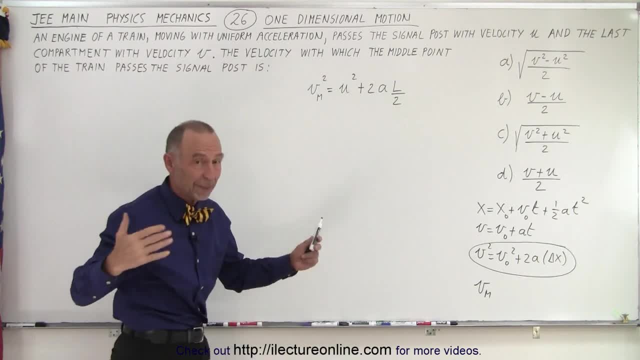 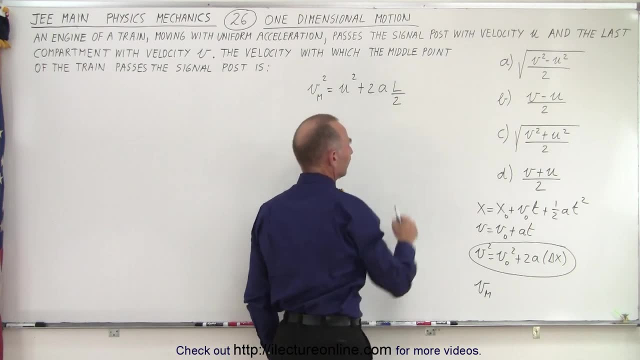 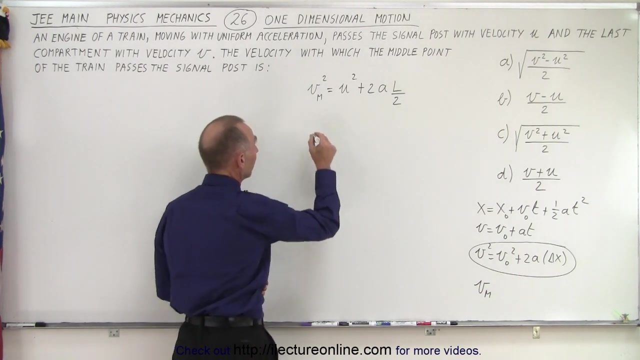 acceleration times, the amount of length of the train. it would be half the train has gone by. But notice that none of the answers include a and l, So somehow we have to eliminate that. So what we could also do is as follows. We could say: well, the velocity at the end of 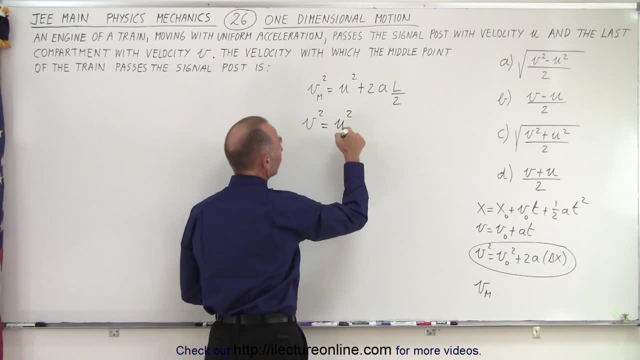 the train squared equals the velocity in the beginning of the train squared, plus two, a times l. So what we can see here is that a times l- if we solve for a times l, because of course the two's cancel out- we can see that a times l is equal to. 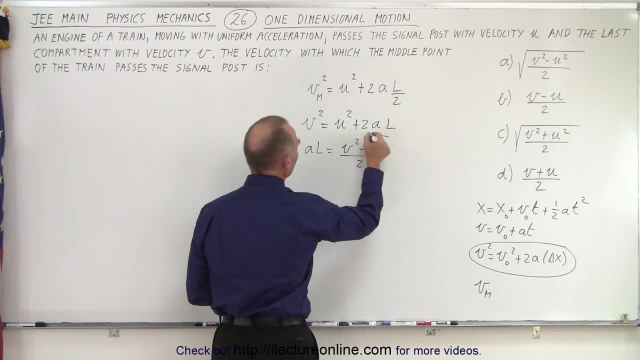 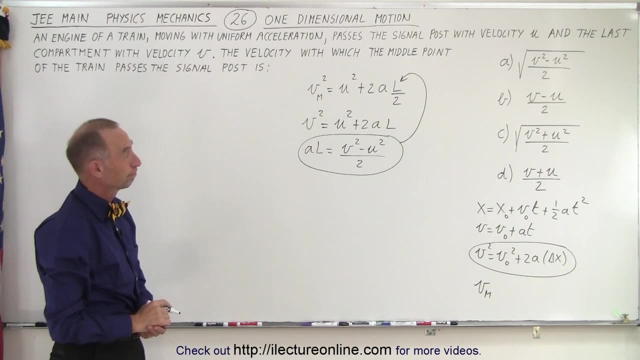 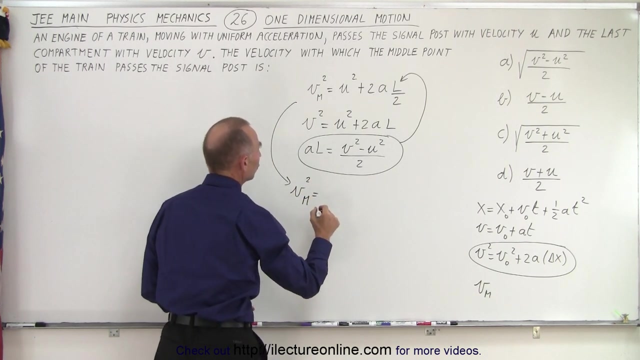 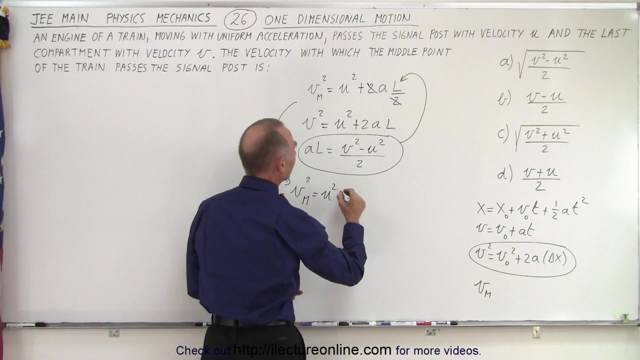 v squared minus u squared divided by two. so this can replace a times l in that equation. so now what we can do is the following: we could say that velocity squared in the middle of the train is equal to u squared, and of course the twos cancel out. like this, and a times l can be written as: 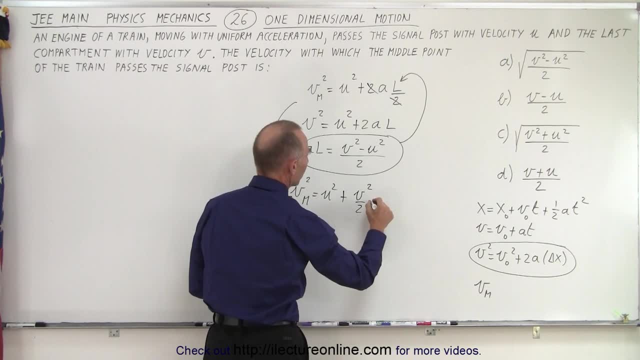 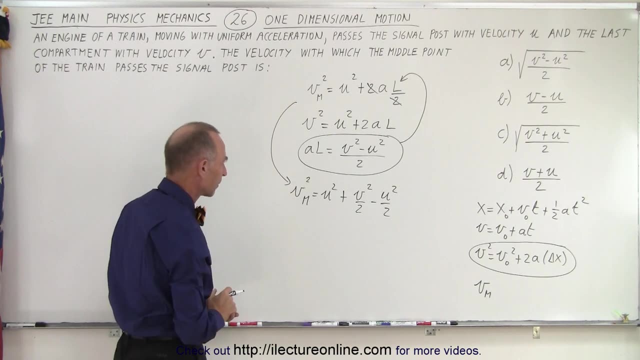 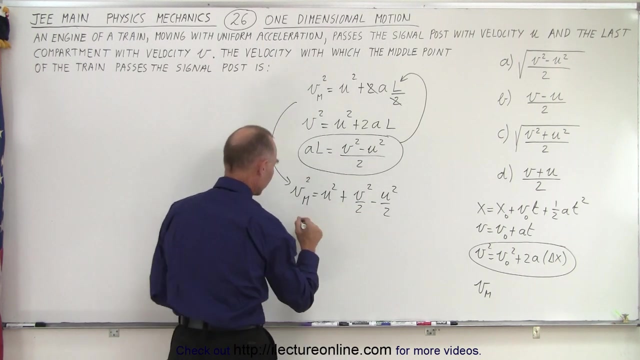 v squared over 2, minus u squared over 2, and now all i have to do is simplify that to find the velocity of the middle of the train. so notice, i have a u squared and a minus a half u squared, so this becomes v middle of the train.